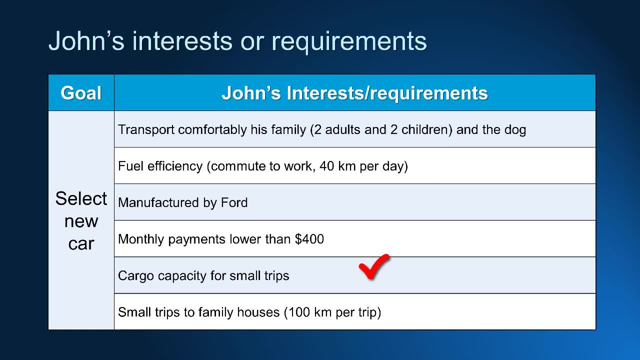 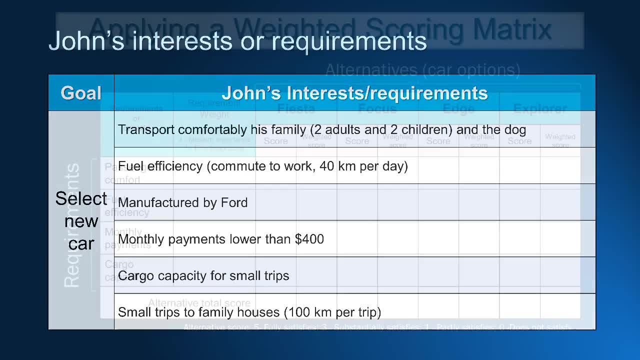 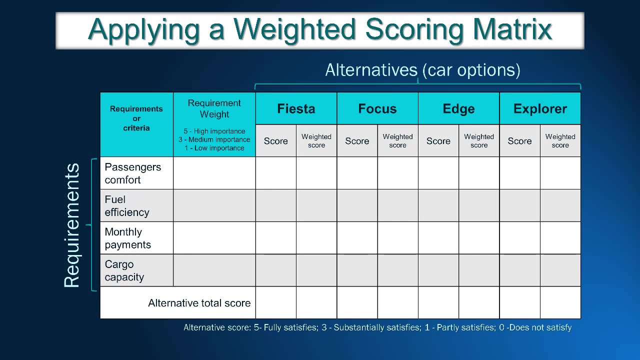 John needs a car to drive every day to work And monthly they visit relatives. that lives 100 kilometers away. It is just a day trip. The first step is to create a table with the requirements and possible alternatives. The requirements are listed in the first column. 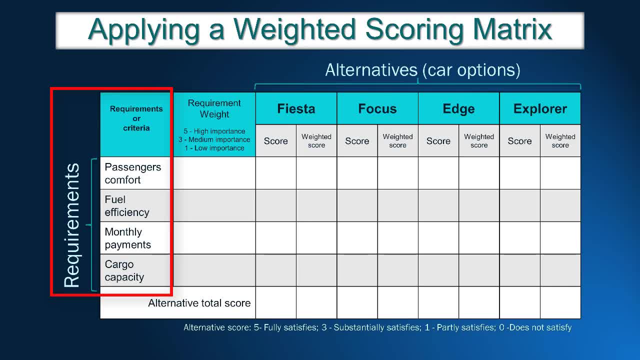 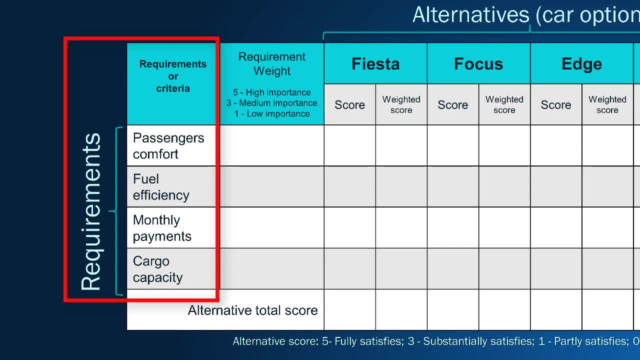 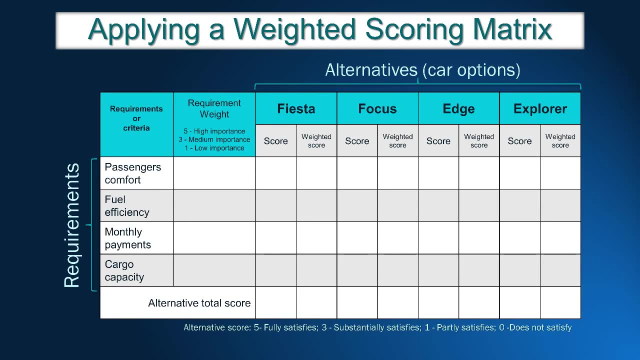 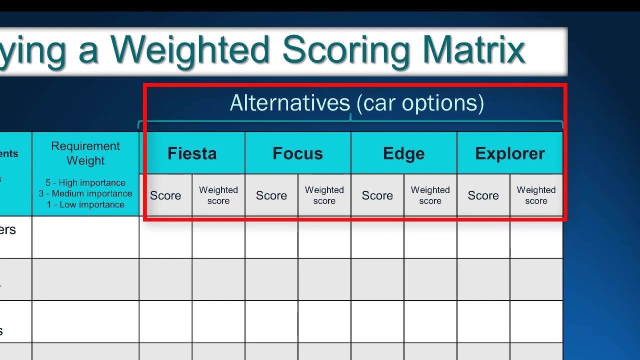 As you can see, we summarized John's needs into four major requirements: Passenger's comfort, full efficiency, monthly payments and cargo capacity. Secondly, we need to identify alternatives, In this case the car models John can buy. To be more illustrative, we decided to present alternatives manufactured by Ford company. 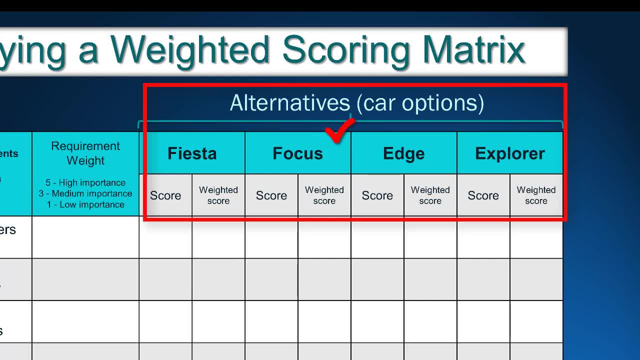 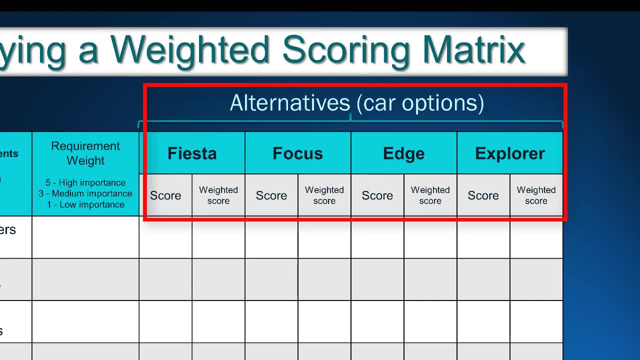 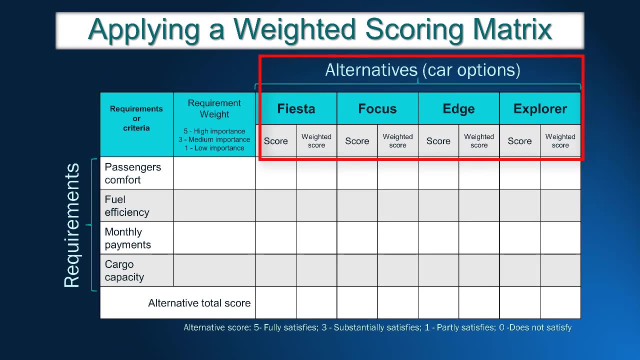 Fiesta is the smallest, cheapest and most full efficient car. On the other side we included the Ford Explorer, a large utility vehicle. In the middle range we have Ford Focus and Edge. Now the weighting and scoring table is ready for the analysis. 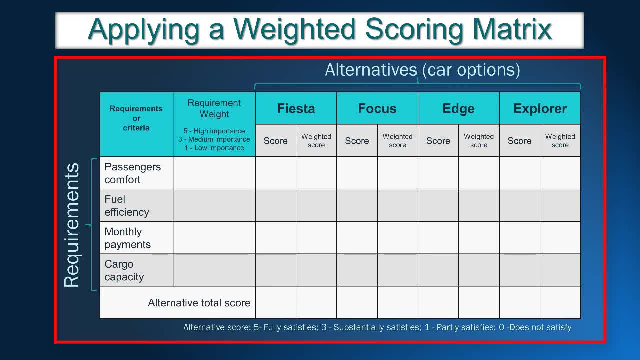 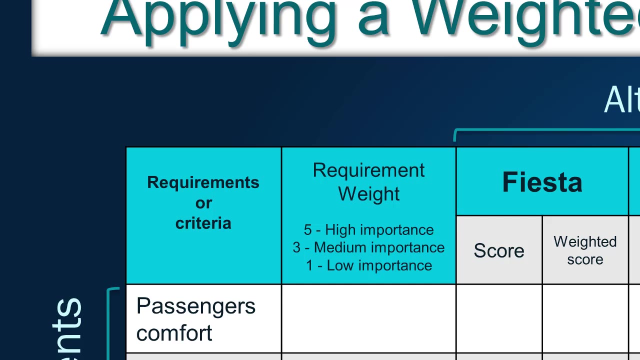 Requirements in the lines and alternatives in the columns. The next step: we need to define the car model. Which requirement is the most important? Which one is the least important? The challenge is to translate the requirement importance into numeric weights. The most important requirement receives weight 5,, high importance. 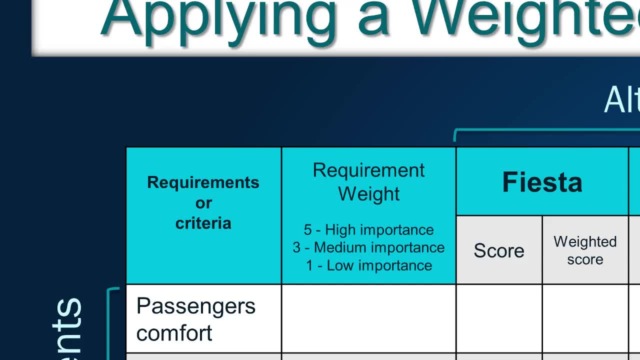 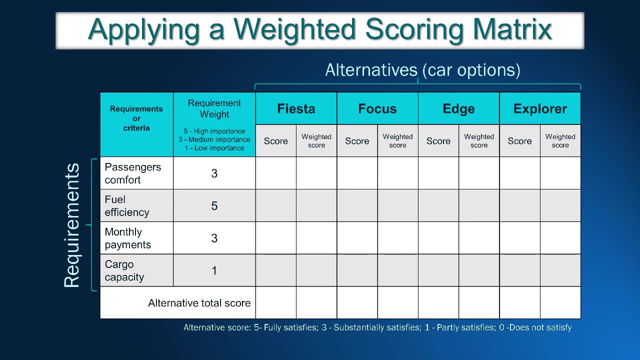 The least important receives weight 1, low importance. Let's make some assumptions for John. Let's make some assumptions for John. John uses his car model. John uses his car model, His car, every day. to work, The vehicle must be full, efficient. 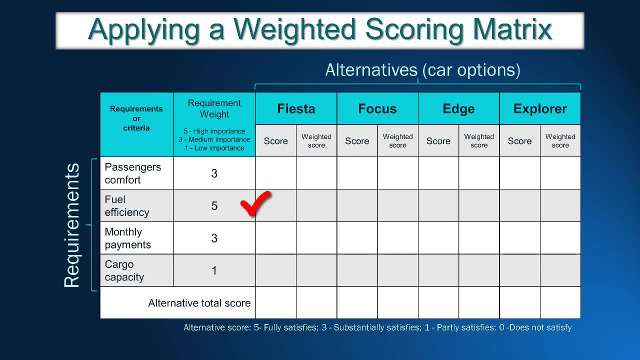 And therefore the requirement full efficiency receives weight 5.. John considers that cargo capacity is not that important and gave weight 1 for this requirement. The remaining requirements receive intermediate weights ranging from 2 to 4.. In this example, passengers' comfort and monthly payments are graded as 3.. 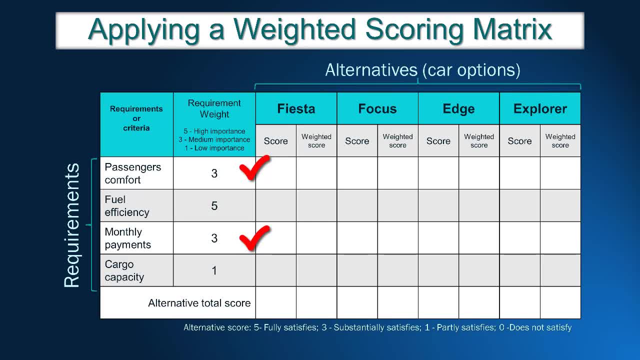 That means that they have intermediate importance in the final decision. In the following step we need to evaluate each alternative on each requirement. Let's start with the first alternative: Ford Fiesta. John thinks that this car satisfies partially the requirement: comfort. John thinks that this car satisfies partially the requirement comfort. Therefore, the requirement for this car is 3.4.. John thinks that this car satisfies partially the requirement comfort. Therefore the requirement for this car is 3.4.. 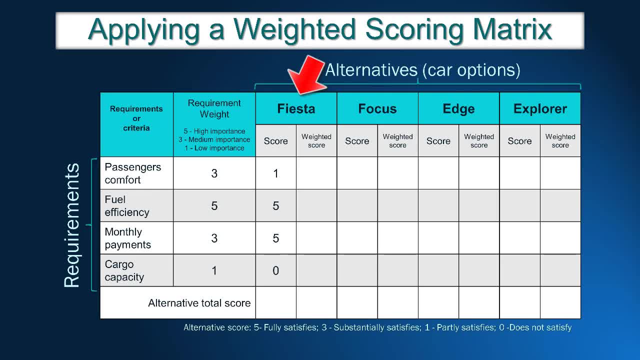 Fiesta receives score 1.. In terms of full efficiency and payment, Fiesta receives the highest score- 5,- because it is the cheapest and has the better full efficiency For cargo capacity. Fiesta does not satisfy the needs And it received score 0 on this requirement. 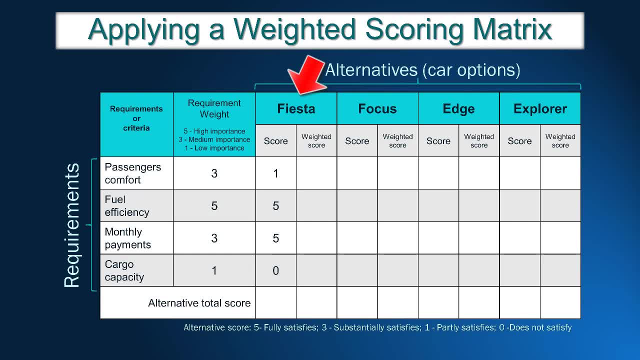 After finishing the scoring for the Fiesta: after finishing the scoring for the Fiesta alternative, John needs to give scores for the remaining models. Once the scoring for all alternatives is finished, it is time to calculate the weighted score. The weighted score is calculated by multiplying the alternative score by the requirement weight. 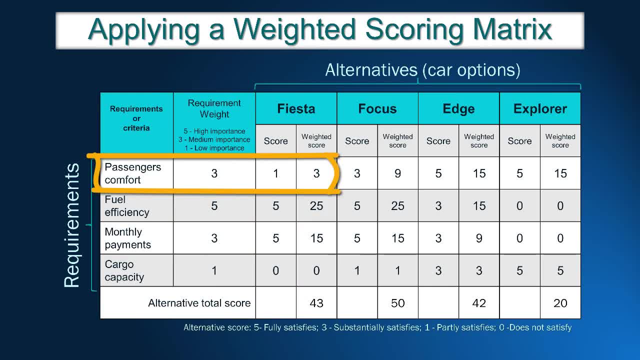 For instance, in terms of passengers' comfort model: Fiesta received score 1.. The weighted score is calculated by multiplying the alternative score by the requirement weight. For instance, in terms of passengers' comfort model: Fiesta received score 1.. The weighted score is calculated by multiplying the alternative score by the requirement weight. 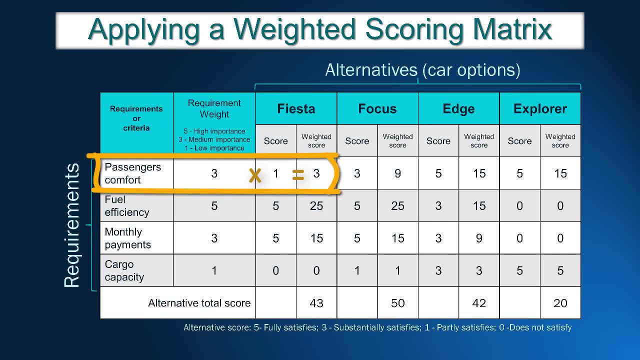 For instance, in terms of passengers' comfort model Fiesta received score 1.. score will be three times one, that is three. for full efficiency, the weighted score is five times five. that comes to 25 after calculating all weighted scores. for the alternative, it's possible. 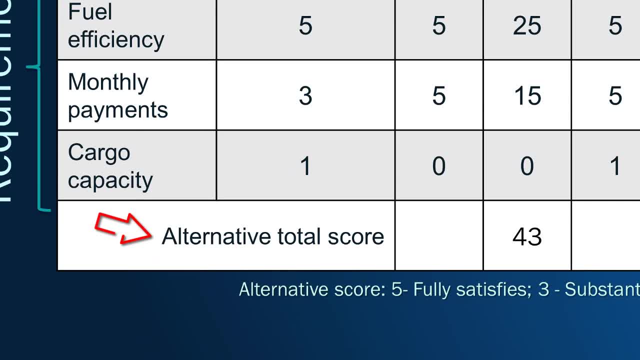 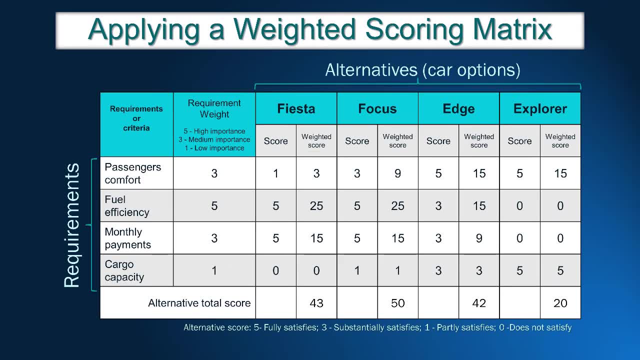 to determine its total weighted score. the total weighted score is obtained by adding up the weighted score for each requirement. for the alternative fiesta, the weighted score is 3 plus 25 plus 15 plus 0. that comes to 43. now we can repeat the calculation for the remaining alternatives. it's: 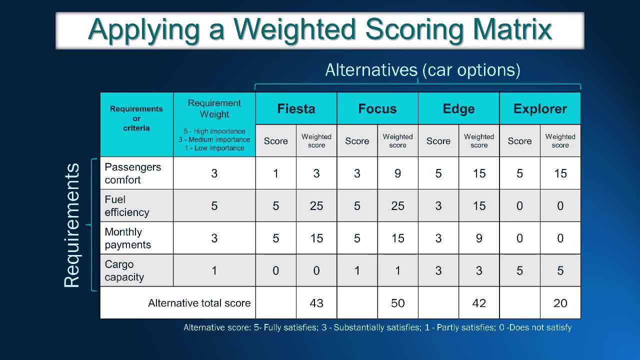 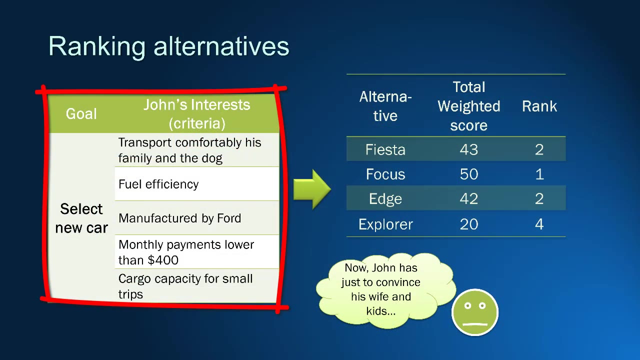 now possible to have an idea how suitable the alternatives are for john's requirements. in fact, the weighting scoring method translated needs and opinions into wages and score, which helps to compare alternatives using numerical values. let's recap: the needs and interests were translated into requirements. the requirements received weights based on the importance level, then the total weighted score. 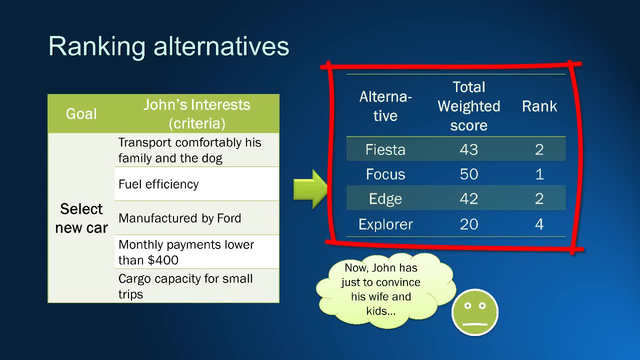 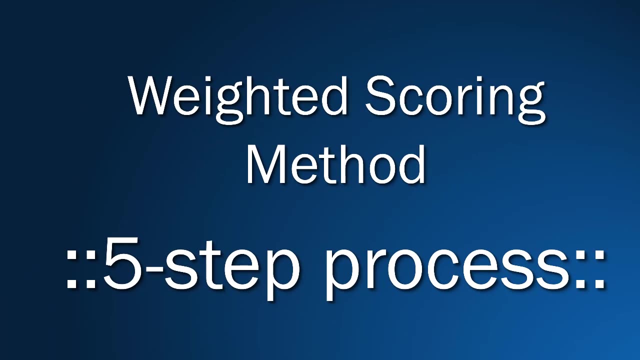 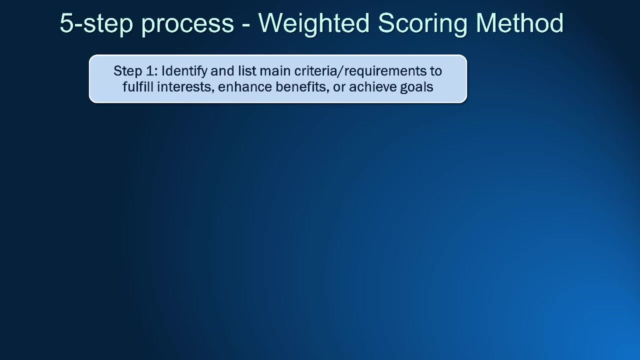 was calculated based on the value calculated following Penelops method. we can first compare height and st magic with wealth, then by intuning the w Eve times and then we'll calculate the measurements that may consist of the weight added price into points and благодарinya. this is the injury part. we're going to 때도 here. in the next video we're going to measure the result in your instrument with weight Norwegian pay note plots made possible to compare and rank alternatives. in this case we may assume that the alternative focus is the most suitable for johns needs. the weighted scoring method can be explained in five easy steps. first, to find the objective and requirements. second, grade each requirement importance with wage. 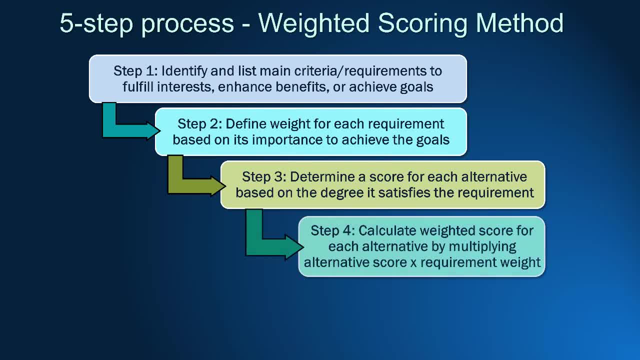 alternatives to achieve the objective. 4. Give scores to each alternative and calculate the total weighted score. 5. Finally, rank alternatives and interpret the results. Let's see the details of each step in the next slides. In the first step, it is crucial to define: 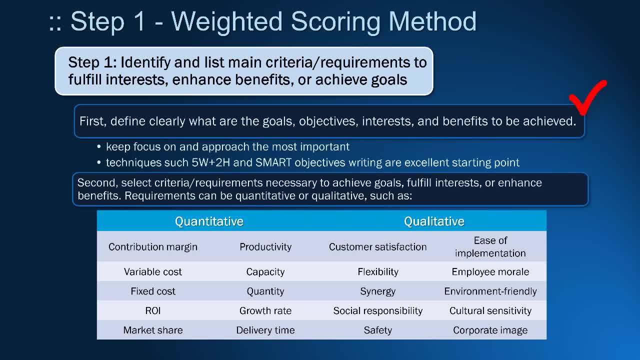 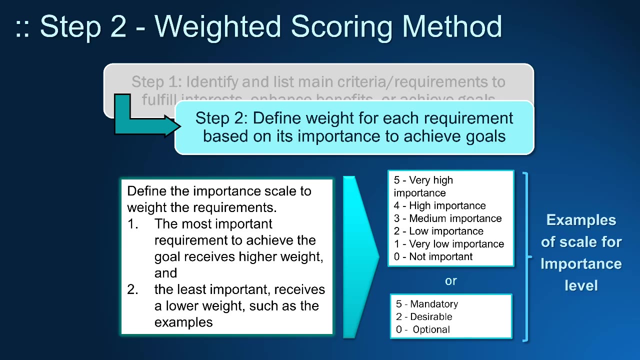 clearly the goal and then choose requirements or criteria that are important to achieve the objective. The requirement or criteria can be qualitative or quantitative. Here you can see some examples for business scenarios. In the step 2, it is time to determine the requirement's importance. Here you have two examples of scale. 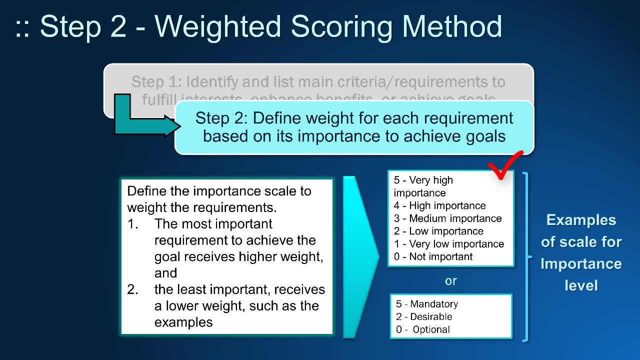 You can use a scale of high to low importance in which you give numerical values 5 to high importance and 1 to low importance. Another weighted scale can evaluate if the requirement is mandatory, desirable or optional. You may give scale 5 to mandatory requirements. 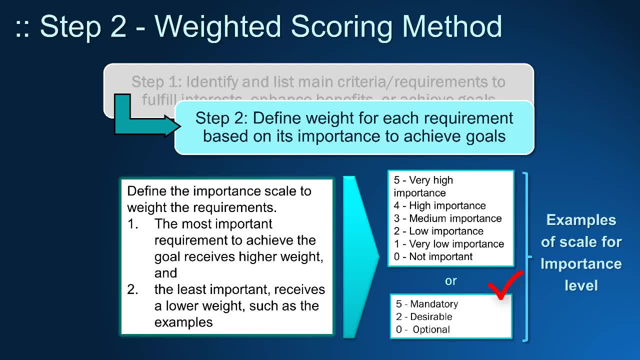 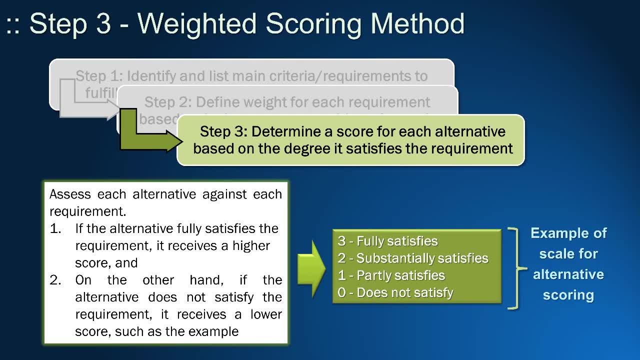 3 for desirables and 1 for the optionals. During the step 3,, you should focus on one alternative of the columns each time and evaluate it on each requirement of the lines. For instance, you may ask: does the alternative? 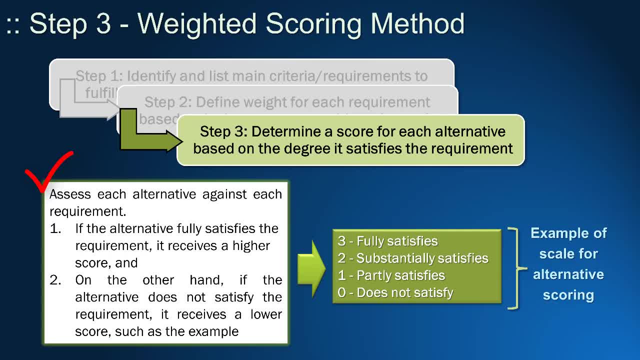 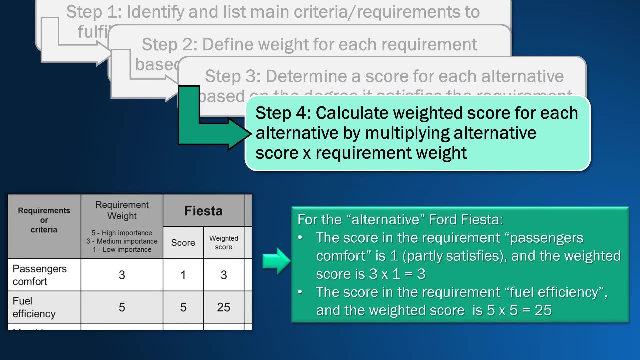 satisfy the requirement. In our example, we could have said: does Fiesta satisfy comfort requirements? The answer will naturally conduct to a score. In the step 4, it is time to calculate the goal. In the step 5, we calculate the weighted score for each alternative by multiplying the score. 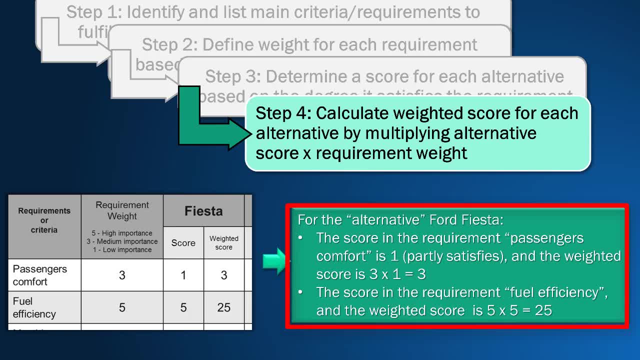 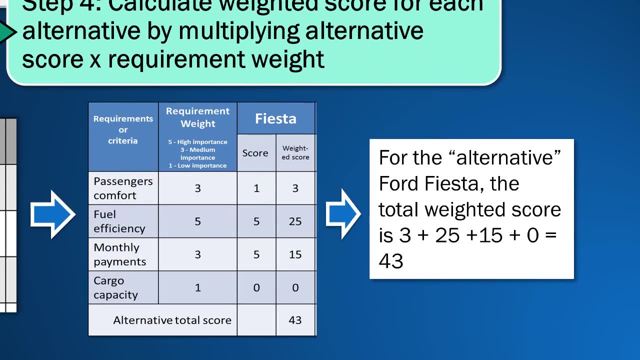 and its respective weight. After determining all alternative weighted scores, we will be able to calculate the total weighted score for each alternative. This can be done by adding up the values in the weighted score column. This is a simple math, as you could see in the example. 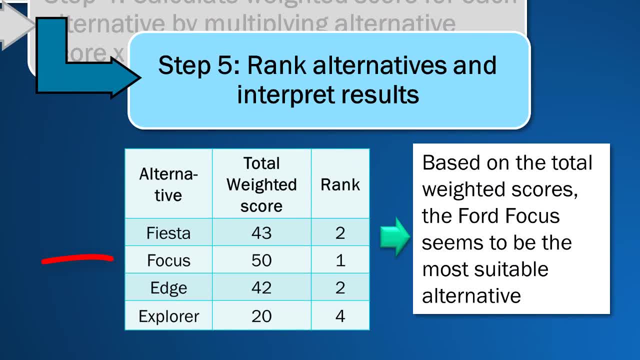 In the last step, you can calculate the total weighted score for each alternative. Next step: we can compare the total weighted scores for all alternatives and discuss the results with the team and stakeholders. In some situations, it can be useful to repeat the method, just considering the three best-ranked. 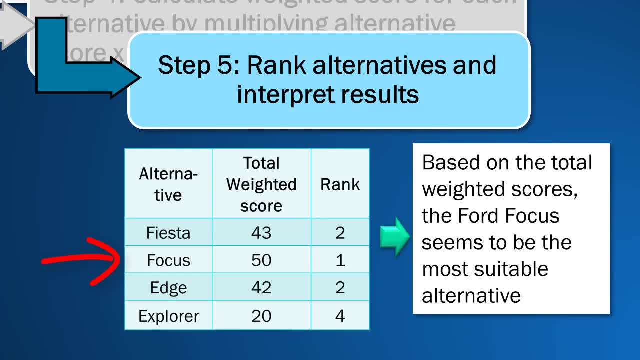 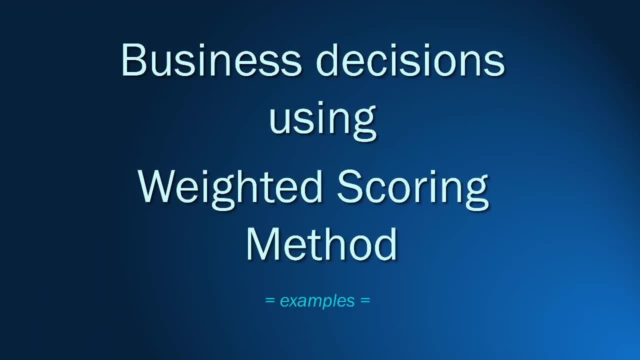 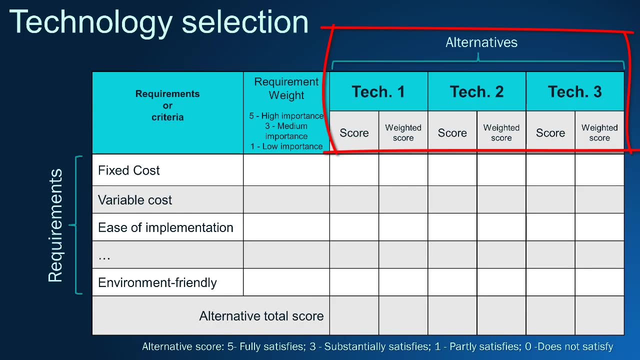 alternatives. By doing this, you will narrow down the focus and increase consistency. Let's check now some practical business applications. This example shows how to select a technology. You can see technological alternatives in the columns and business requirements in the lines. You can evaluate each technology against each requirement and then identify the most suitable. 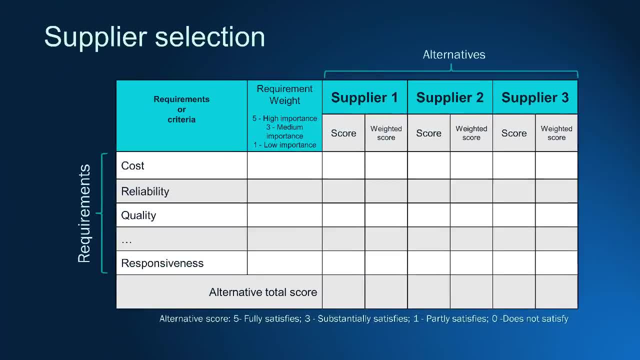 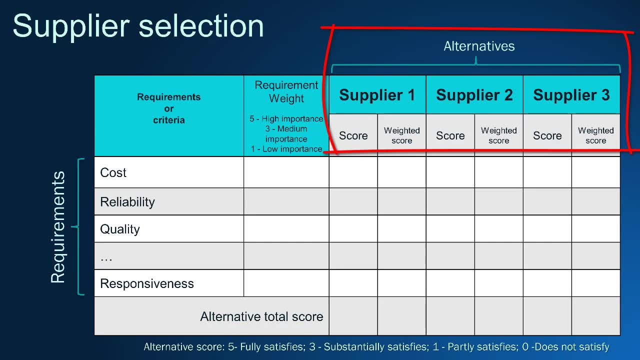 for a specific application. This example shows how to approach a supplier selection. The suppliers are placed in the columns and the company business requirements are placed in the lines. By providing ratings for each supplier, you find out the best supplier to provide the resources required.